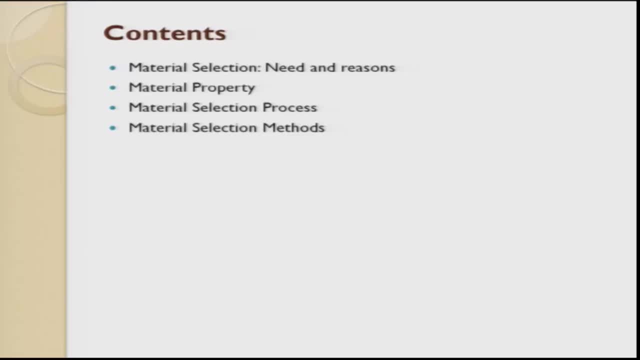 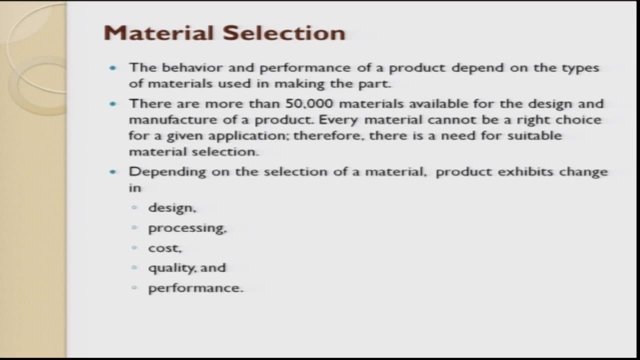 is the need and reasons. next, what are all the material properties, the material selection process and the material selection methods, what we follow here? So material selection is, ah, very important ah. So here what we do is we try to take the behavior and the performance of the product. 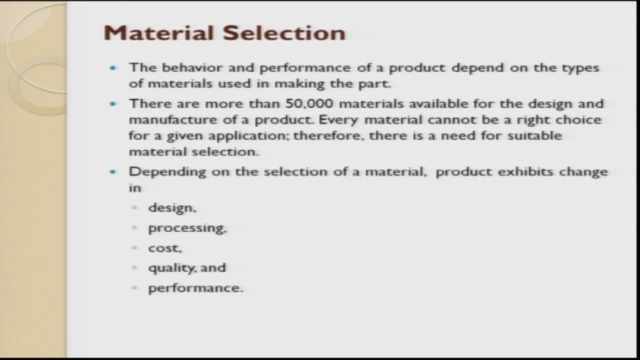 both depending upon the type of material which is used for making a part. For example, a chair can be made out of steel, a chair can be made out of wood, a chair can be made out of polymer material. So what does a customer want? 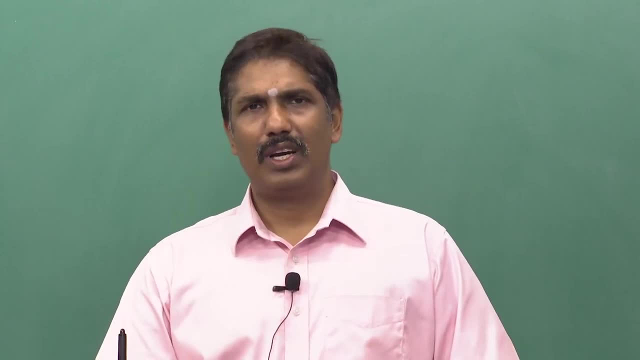 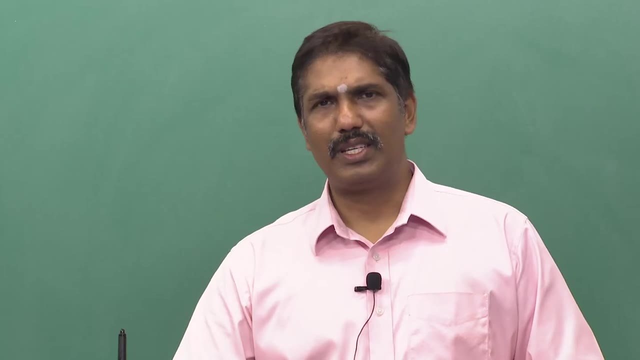 A customer. as far as a customer is concerned, he is more ah comfortable. he looks for a comfort to sit in a chair. Second thing: after ah the event is over, ah, the supplier or the, even a customer, would like to have a stacking sequence such that he can store after the. 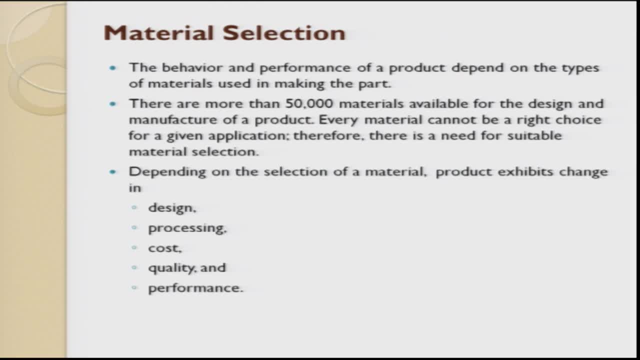 event is over in a very short place. So these are the two requirements. generally we have a customer For doing this. you can choose. Choose wood as a starting material, steel as a starting material and plastic as a starting material. Polymer does not corrode ah in due course of time, So polymer has a longevity. 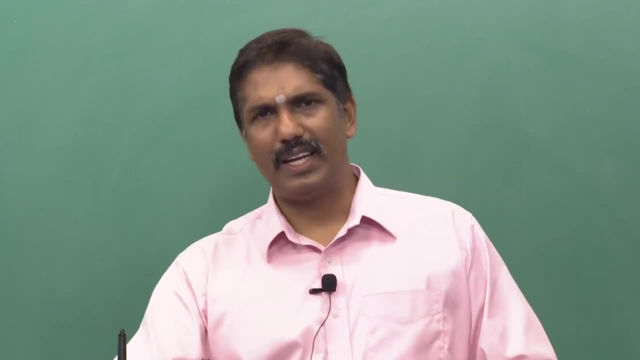 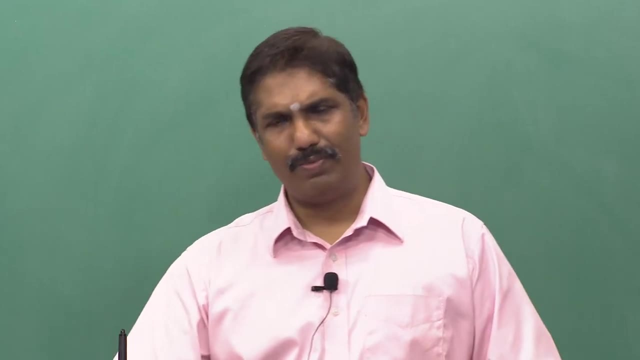 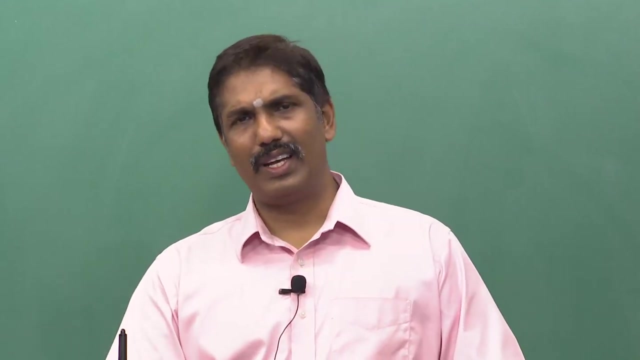 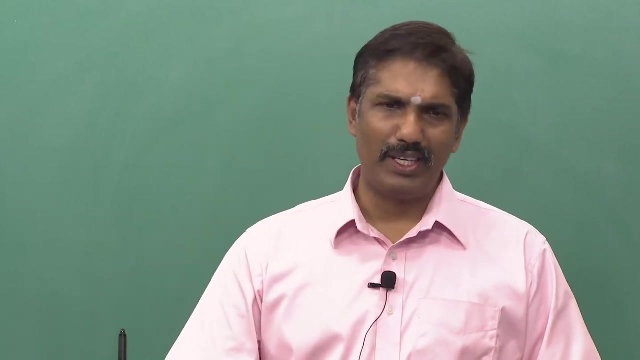 in in work, The wood based and the steel based. they always have a environmental influence on the product And over a period of time they both get deteriorated very fast. So both the steel chair as well as the wood chair has think of a folding process and then stacking it together. but the only thing is when you 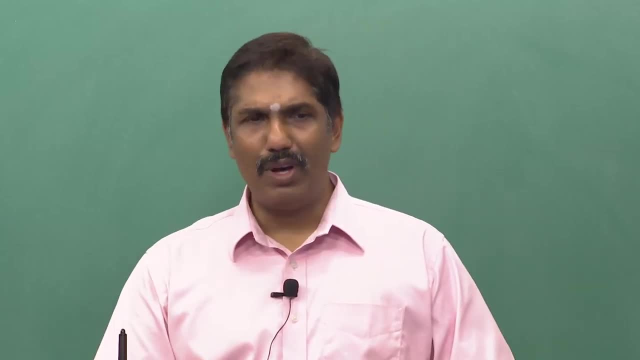 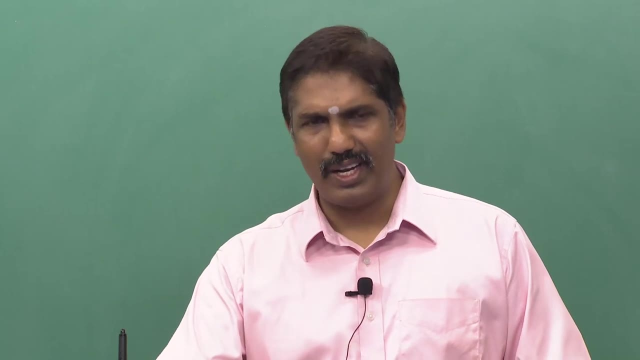 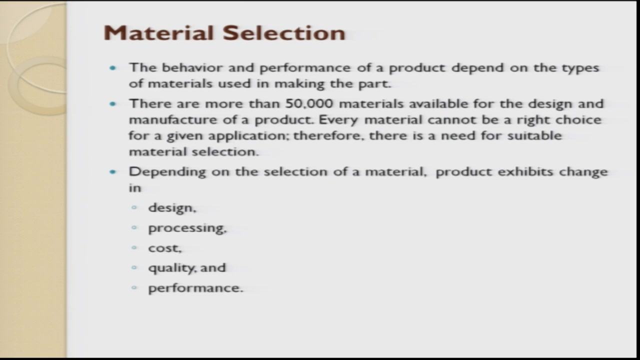 work with steel or when you work with wood, the number of parts which are involved for assembling and making a chair is very high. So the assembly process is very high. the maintenance cost is also very high. Now, keeping all these ideas, we have supposed to choose a particular material When we choose a particular material. keeping all these, 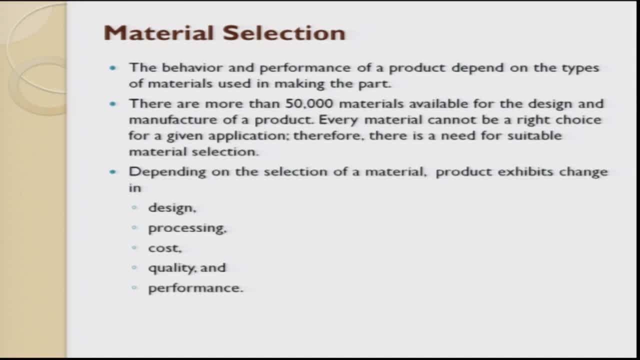 things prerequisite, then what we do is we choose a material. then, corresponding to that material, we choose a process. In fact, there is one more important aspect in all these choice making is the cost. what is the cost I give for that product? So keeping all these things cost mechanical properties and other endurance properties. 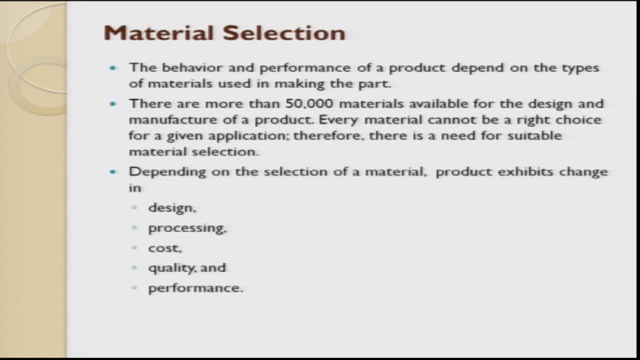 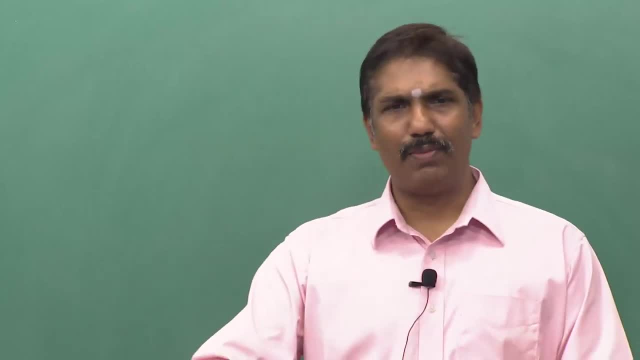 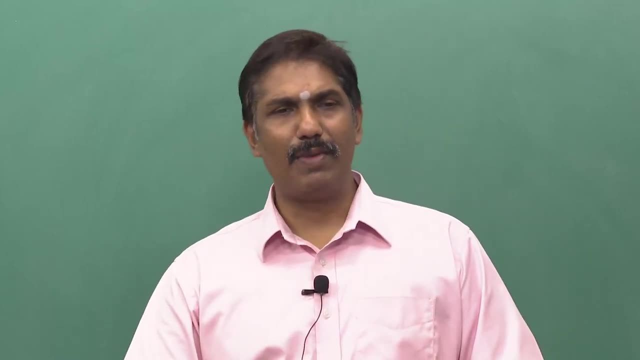 into into consideration. we have to choose a material so that we make the customer happy. So here the first: the behavior and the performance. performance is how good the product performs or how happy is the customer. So performance of a product depends on the type of material used in the product. 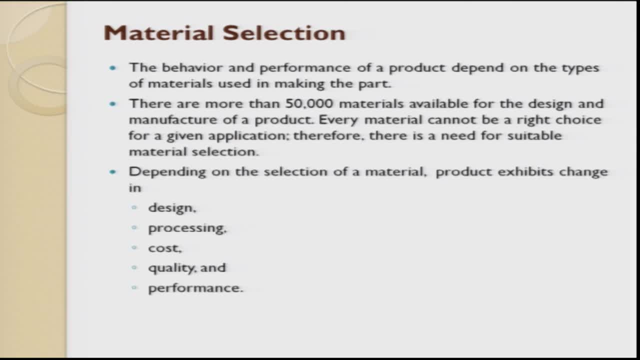 There are more than 50,000 materials available for design and manufacturing of a product. today The spectrum is very large. Gone those days. you have only 3,000.. 3 parts, 4 parts or 4 different materials. we choose that and start making it. 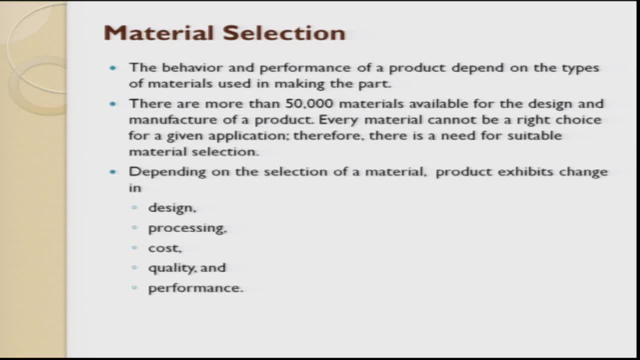 People thought this part, which is a structural component- this has to be made out of steel- is now replaced by polymer matrix composite. The weight has gone down, the performance has enhanced and, as far as polymer, we have already known that, depending upon your requirements, you keep adding ingredients to meet out your 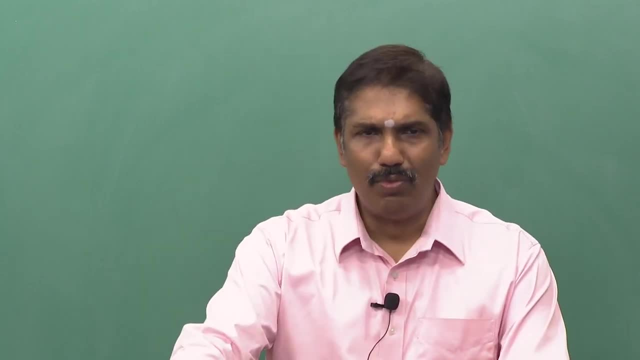 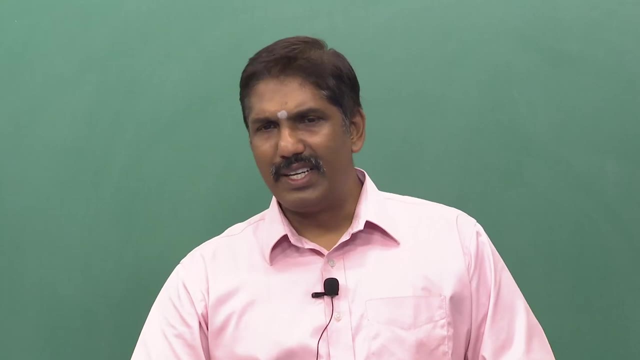 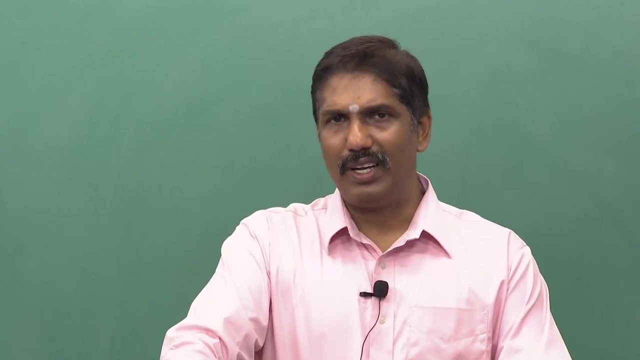 ah properties. So there are more than 50,000 materials available. More than 50,000 materials available for design and manufacturing of a product. Every material cannot be a right choice for a given application. Therefore, a suitable selection has to be done or an optimum selection has to be done for. 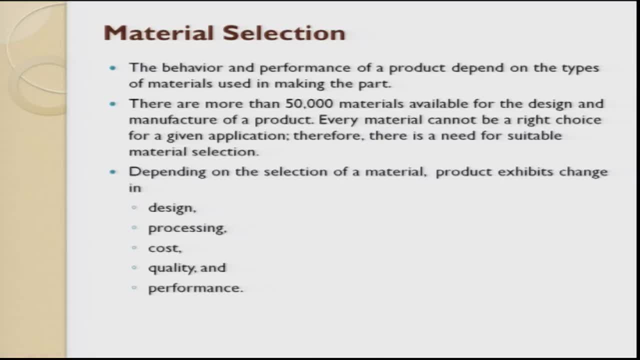 choosing a material. Depending on the selection of a material, the product exhibit changes in design, processing, cost, quality and performance. Interestingly, the shape of the product can be changed to meet out the requirements. For example, if you think of having a square shaft, it can be made circular, keeping manufacturing. 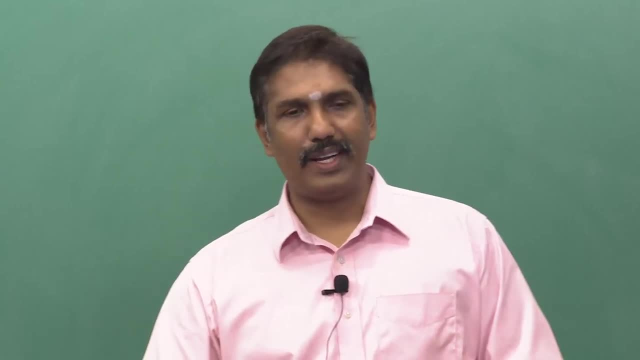 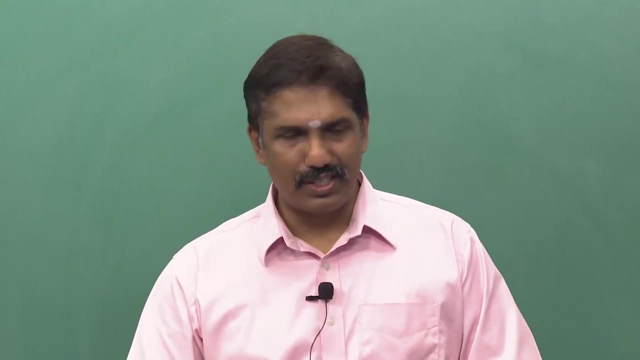 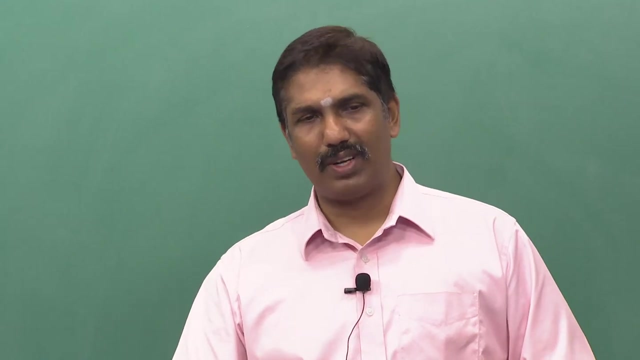 as a important weight, giving more weightages to the process. we can always make it cylindrical. Earlier square sections or rectangle sections- box sections- were thought of very was thought to be very difficult in manufacturing. Today there are lot of new process and process ease has happened. 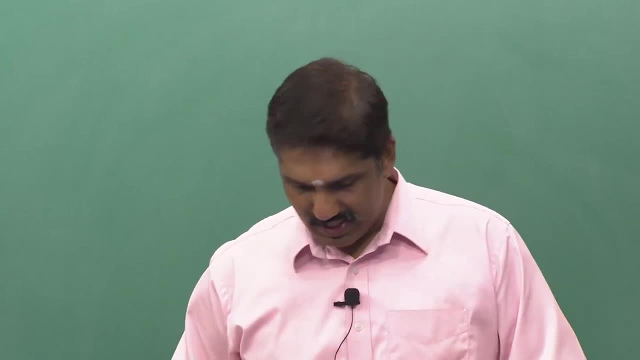 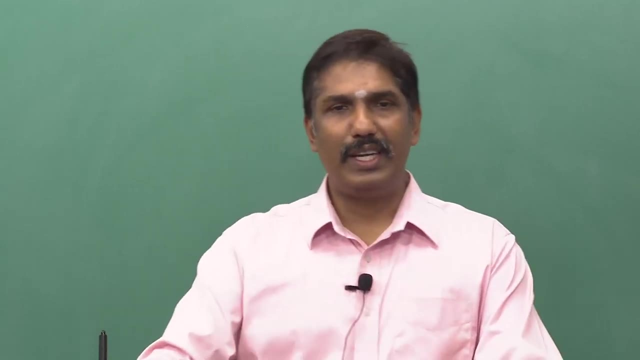 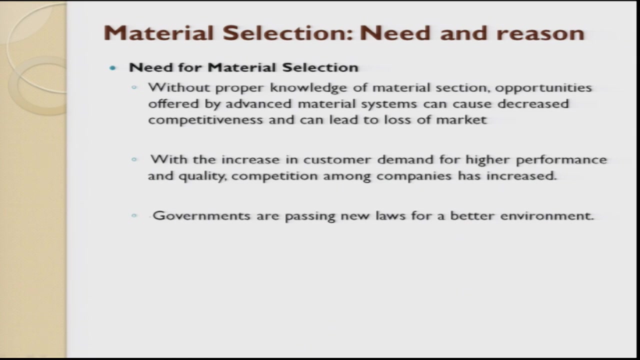 So we can design any component and we can manufacture the same. So what is the need and reason? So the need for material selection. without a proper knowledge of material selection opportunities offered by advanced material systems can cause decreased competitiveness and can lead to loss of material. 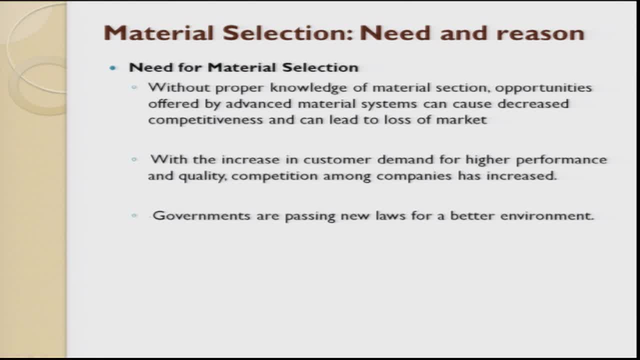 So if you make a wrong choice- For example, sensors were initially thought of to be made by glass, then they moved to silicon and today they are made out of polymer. Polymer is lightweight, roll to roll manufacturing can be done very easily. So if you do not have the proper awareness, knowledge about the material selection, then 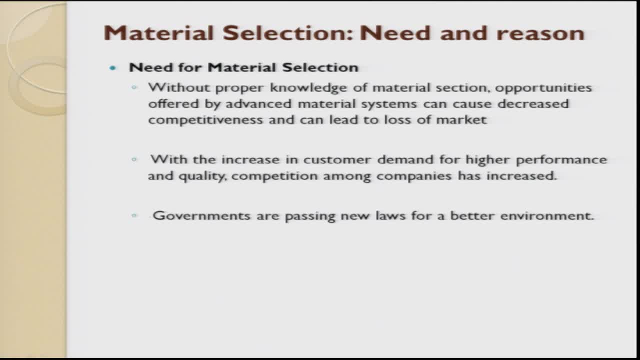 you will not be able to push your product or your product will not be much successful in the market With the increasing of customer demand. So today we are not able to push our product. Today customer has is becoming more and more demanding. So what he wants is he wants a very lightweight part which can do multiple operations or processes. 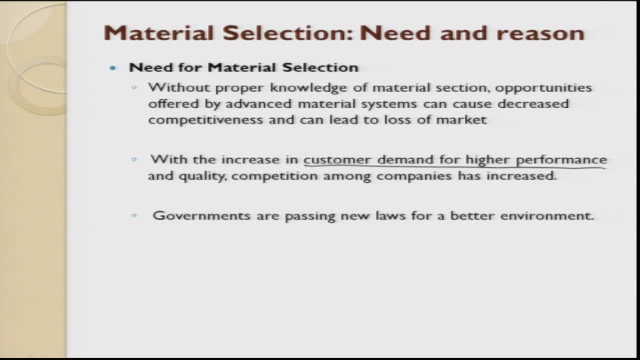 and which is having very low maintenance with a low costing. So you see, all these demands which customer puts in front of manufacturing is all contradicting to each other. But still he says I will give you this much price. So that means to say he wanted to buy the product in a very, very economical manner. 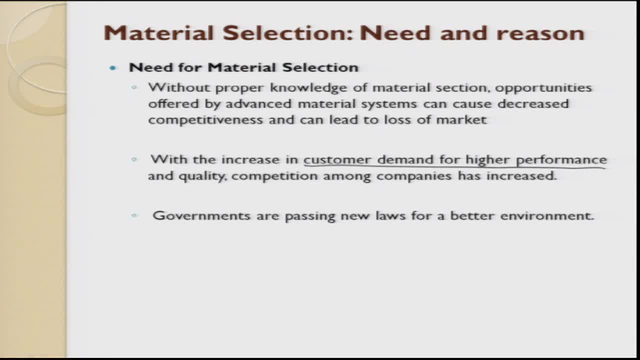 So the customer demands for high performance and quality and competitiveness among company has increased. So a proper choice of materials is very, very important, And today the government norms have also become very stringent. They are now talking about a green earth, So where in which the material which has been chosen for making a product, what the government 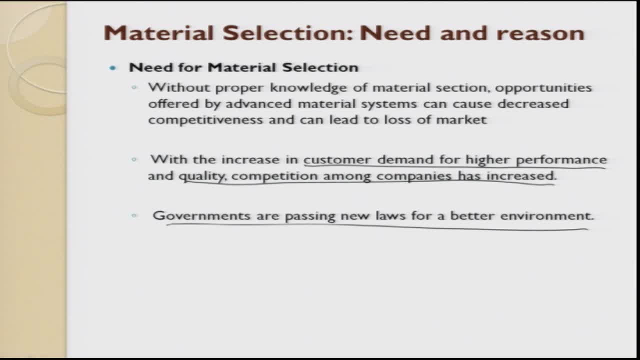 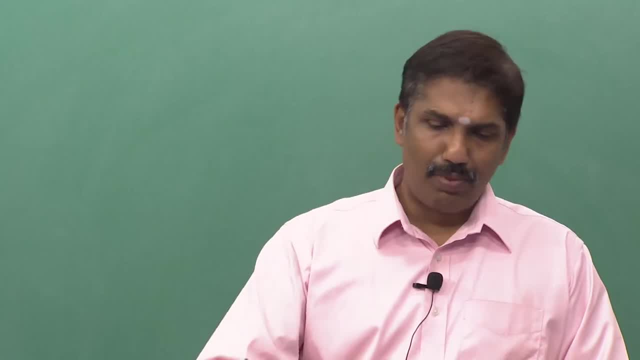 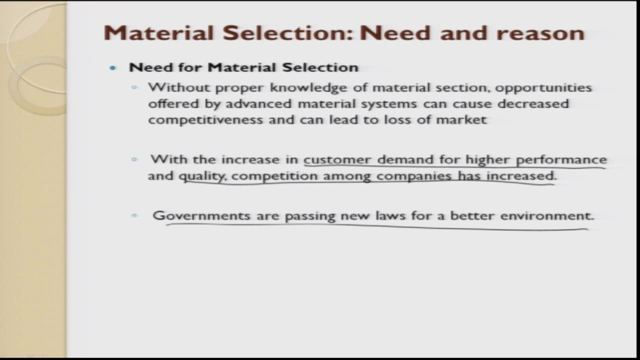 norms are pushing very hard is it should have minimum carbon footprint, It should be biodegradable or it should be recyclable. So these things put a huge demand on the designer to make a proper choice or to make a selection, material selection proper to achieve the product. 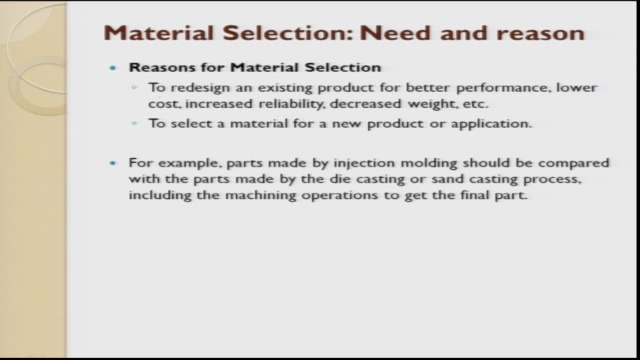 So the other two points which are very important: One is to redesign an existing product. So whenever a product is made, if the product is made out of a material- which is the ultimate- which cannot be recycled, which cannot be reworked, then there is a huge problem in 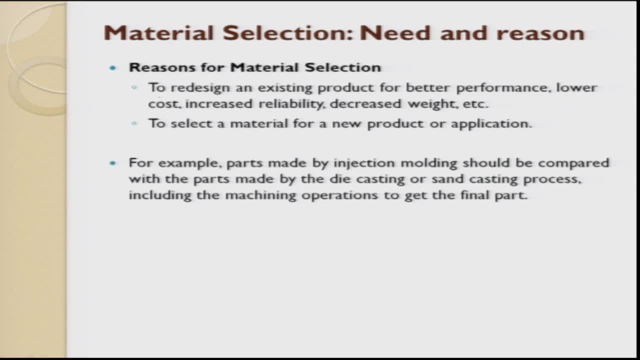 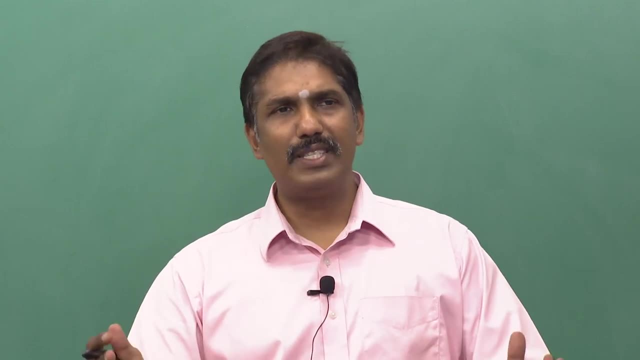 those materials. So today, what is happening? the designer is told that please give a small window such that we can try to redesign or redefine the product such that it can meet Okay Customers or it can be made to meet to a set of customers. 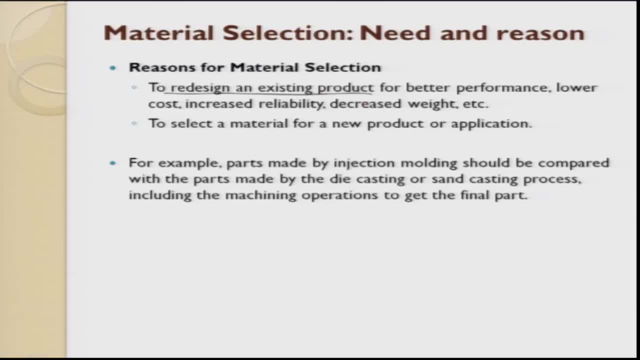 So to redesign an existing product for better performance, lower cost, increased reliability and decreased weight. decreased weight, etc. are some of the reasons which push for material selection. So to select a material for a new product, we always have to do material selection. 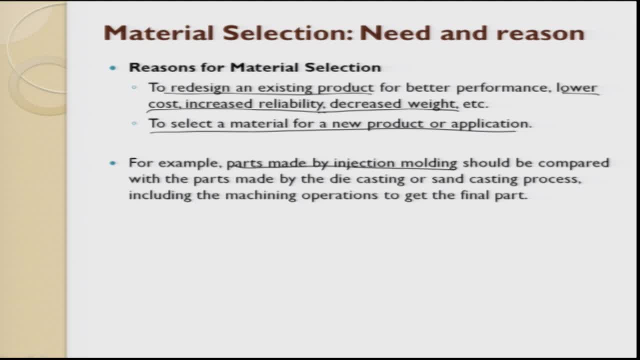 Let us take an example. A part can be made by injection. molding should be made. Okay, So what we have? Let us take a simple example of wheel rim which is used. So earlier days these wheel rims were made by casting. The same wheel rims today are being made by pressure die casting. and these wheels today 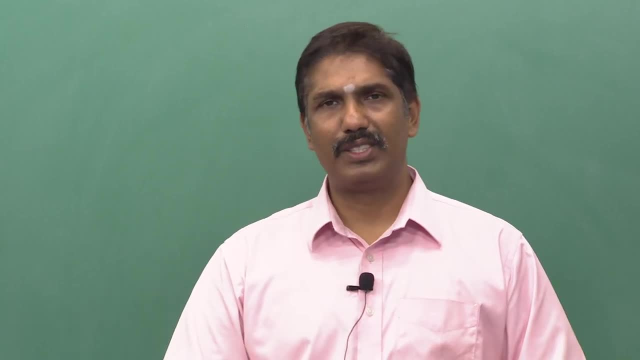 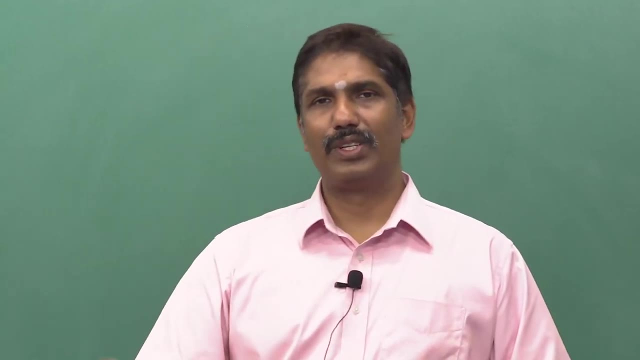 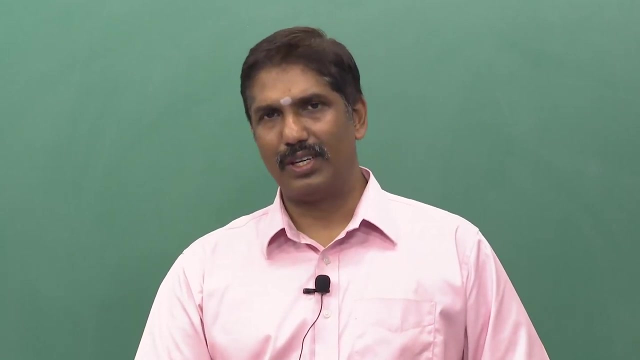 they are being added more reinforcement using carbon fibers and other things, and they are thinking of making these wheels by injection molding process. So basically it was initially cast iron, From there they went into aluminum- lightweight, high strength and mass production, was batch production was done and from there they are now trying to move to injection molding process. 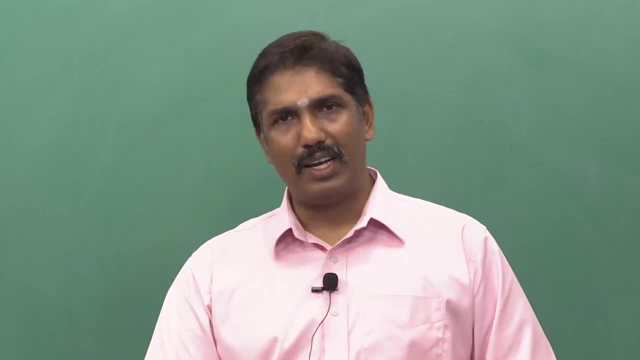 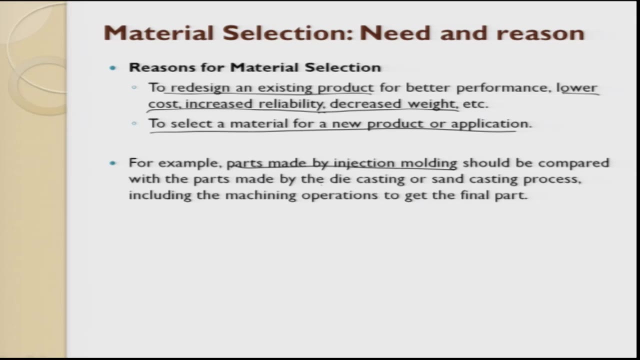 keeping polymer there, reinforcing with carbon fiber, making it light and making it high performance, such that they can be doing a better performance to the customers. So, for example, if you have a wheel rim to be made, this can be made out of the three choices. 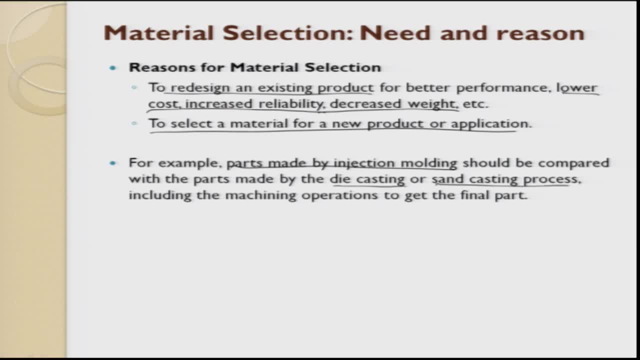 One is casting process. It can be made by die casting process Or it can be made. today they are looking at injection molding process. So injection molding process, polymer is used and the carbon fibers. I said the carbon fibers can exist in several forms. 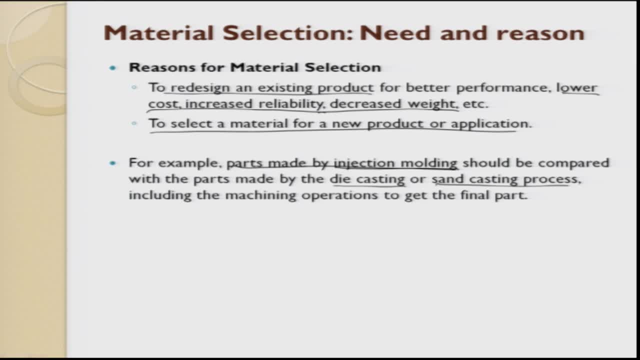 So they try to make a three dimensional reinforcement and inject polymer into it and where in which they are also thinking of placing a location for inserts. So this is what it is. So when casting process was thought of, there was lot of machining operation, which was a 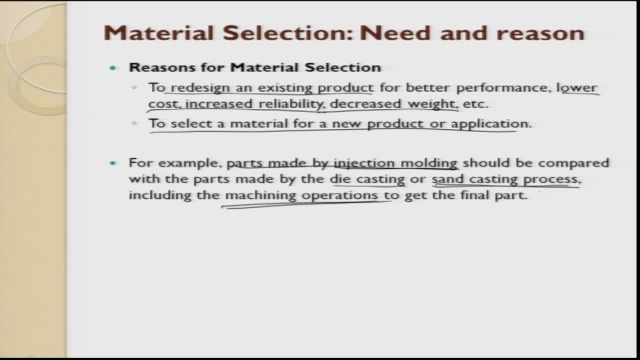 lot of work included. We were not able to make ah, near net shape process, near net shaping, which is the big advantage of polymer matrix composite. So this was not been achieved. by sand casting process. When it came to die casting, yes, we were able to make, and when it goes to injection molding, 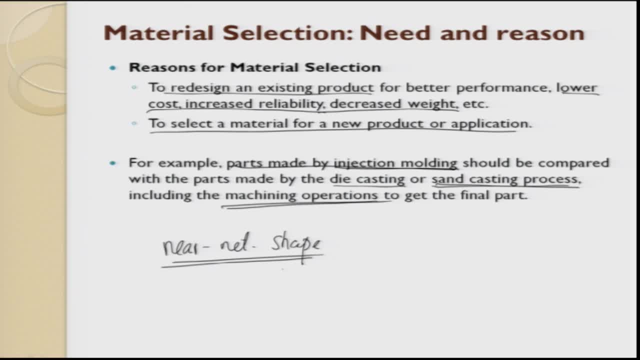 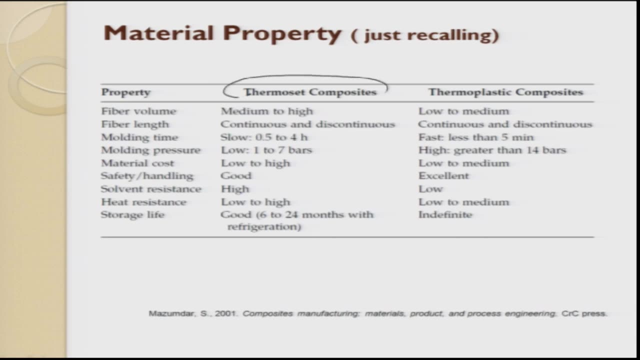 we go very close to the final product itself. So for doing this, you should have a proper knowledge about the material selection- Yes, The material selection for the product. So this is just a recap. You can see that we saw about thermosets, thermoplastic, composite thermoplastic, the. 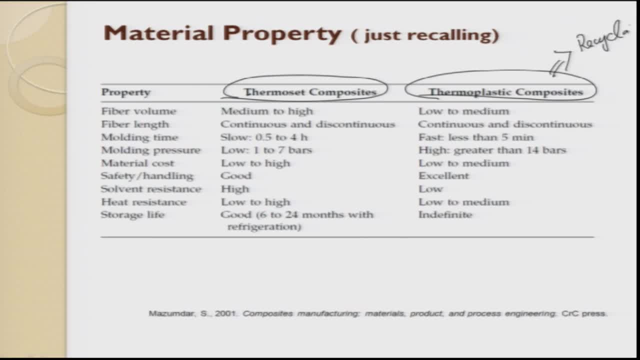 major thing is recyclable. recycle, But here it is non-recycle. The fiber volume fraction: it can go from medium to high, It can go from low to medium, Why? Because when you keep a preform and the, the matrix, if it is in a liquid state, so it can. 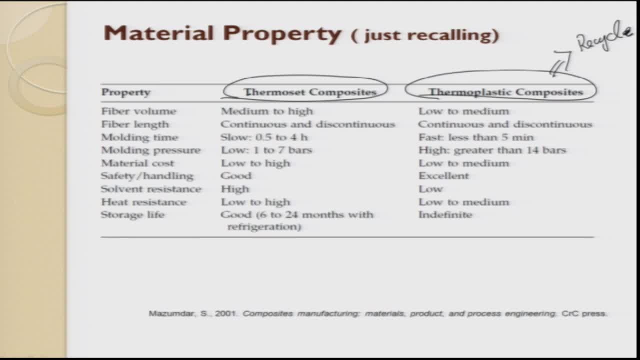 easily flow and try to take a shape. But whereas in thermoplastic you always apply a pressure, where in which you keep a preform of reinforcement and you apply pressure and then push it inside, So you cannot go more than medium. So here you can go to as high as 80 to 90 percentage. 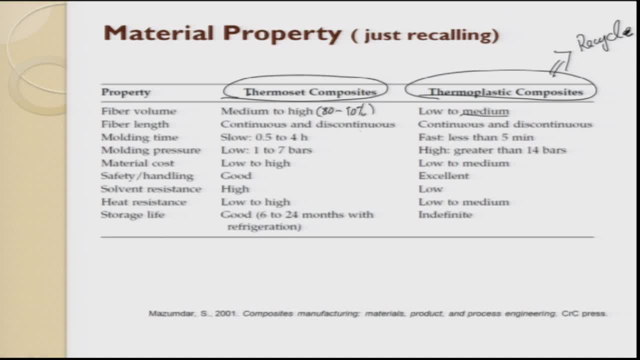 So here the fiber length can be continuous, It can be discontinuous. Predominantly here it is discontinuous. Today it is getting more to continuous. The mold time in thermoset is somewhere close to 4 hours, But here you see, it is less than 5 minutes. 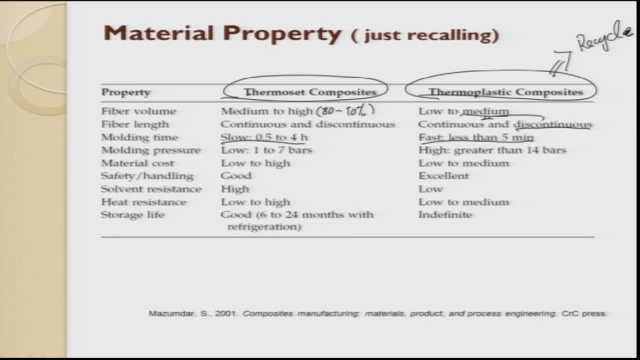 So if you are looking for mass production, then thermoplastic composites are very good. So the pressures which are involved is 1 to 7 bar. We will see where is this pressure. This is used in thermoset when we talk about manufacturing of composites. 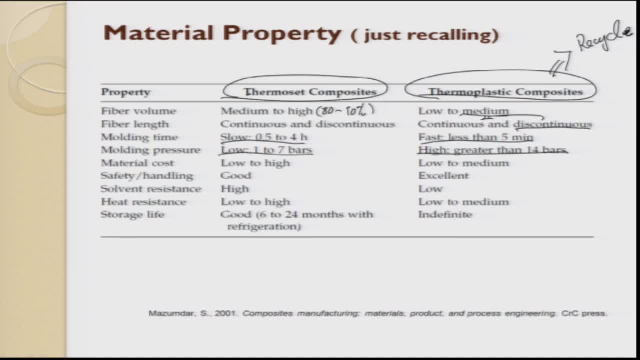 Here the pressures are very high. So when the pressure is very high, what happens? it is a viscous fluid flowing and then you have a preform already laid there When you inject it at a higher pressure. since it is a viscous fluid, the preform can move. 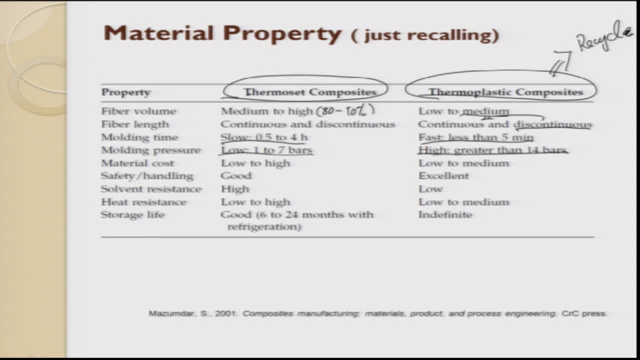 So it is very difficult for you to hold the preform and then inject it, If at all. you put a spacer, that spacer becomes an integral part of the composite spacer or a holding device. Material cost is low to high. It is low to medium. 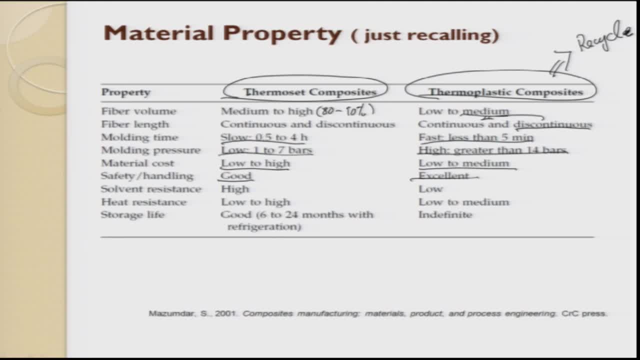 Safety handling is good. It is excellent because predominantly thermoset thermoplastic polymers are solid. They are available in pellet form. They are also liquid form. The solvent resistance is very high. The solvent resistance is low because the material can be etched if you use for acid. 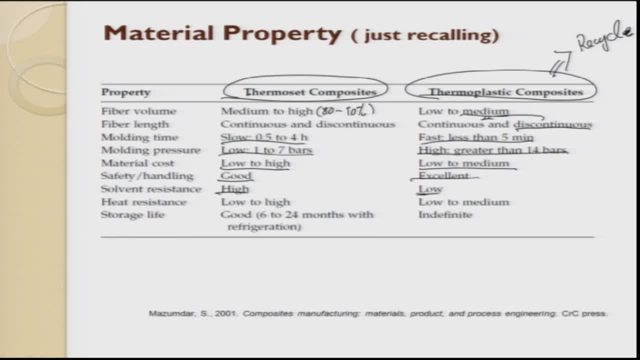 applications. But whereas if you choose a proper thermoset it is very high, Heat resistance it is almost the same because it is a polymer material, So it is very high. The storage life is very good and it is indefinitely, So that means to say it can be there for any time. 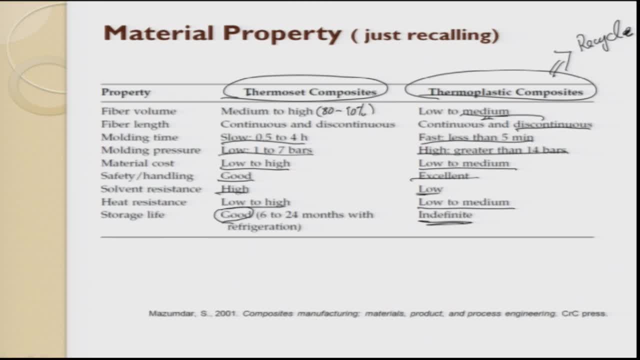 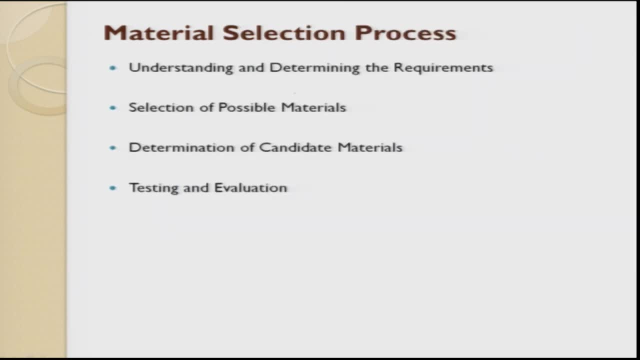 So this is a recap which we already saw. So these are some of the properties you should know before making a choice for making a or fabricating a composite. So the material and selection process can be now divided into 4 things. One is understanding and determining the requirements. 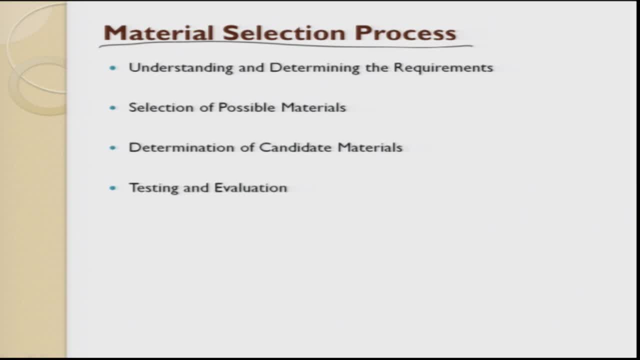 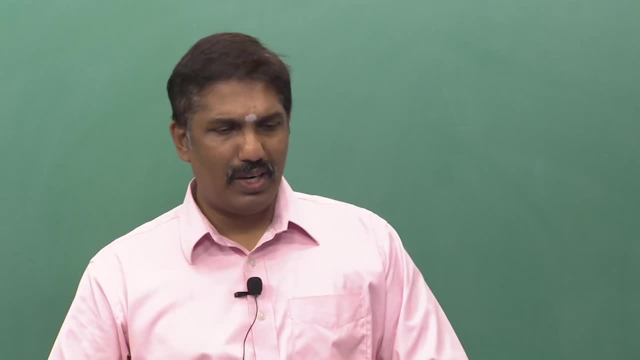 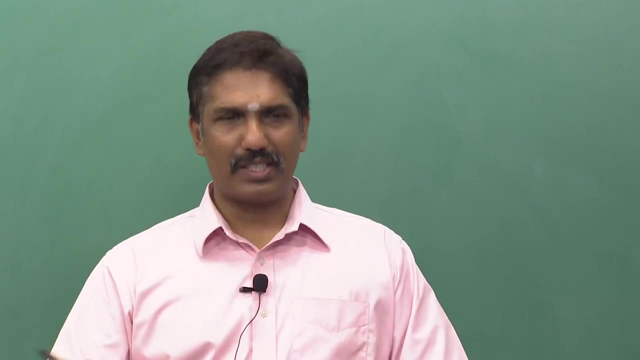 Empathy. that is the biggest problem As a manufacturing engineer. we many a times do not understand the customer's choice or the customer's requirements. So that is what in design process. they say: please do an empathy study. So empathy study means you become a customer for the product and you list down what do you. 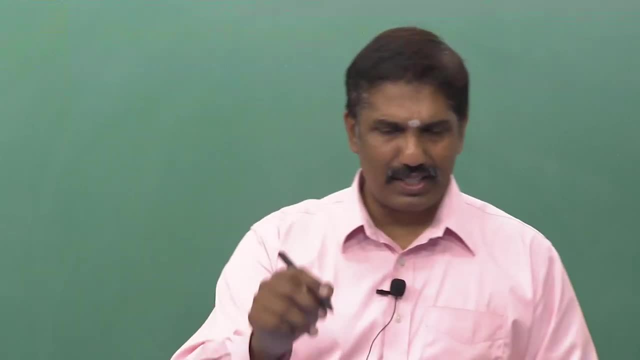 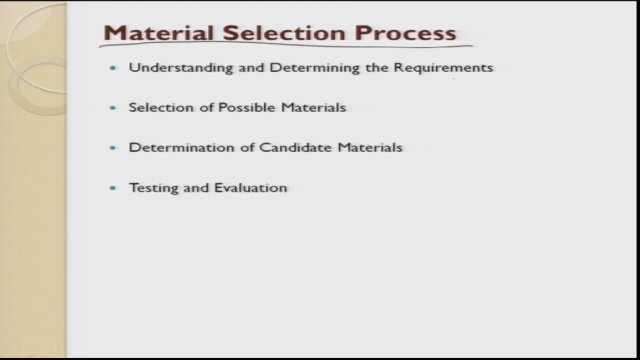 expect from the product. So the material selection process first starts from what does a customer want? So understanding and requiring the requirements. So the material selection process first starts from what does a customer want. So the material selection process first starts from what does a customer want. 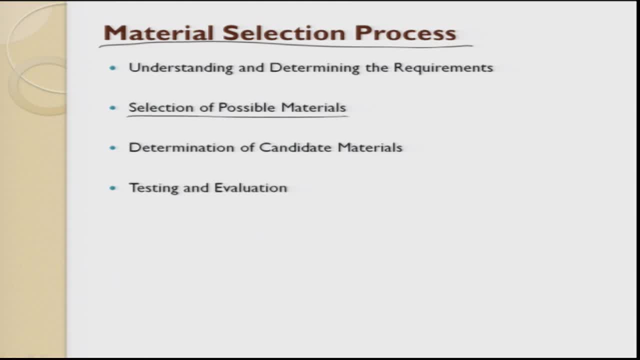 So, understanding and requiring the requirements, Then you make a selection of a possible material. Then what you do is: then you make a determination of the candidate material, Then you do a testing and evaluation before the product goes into the market. So here, first you understand the customer, then you try to select all possible so that 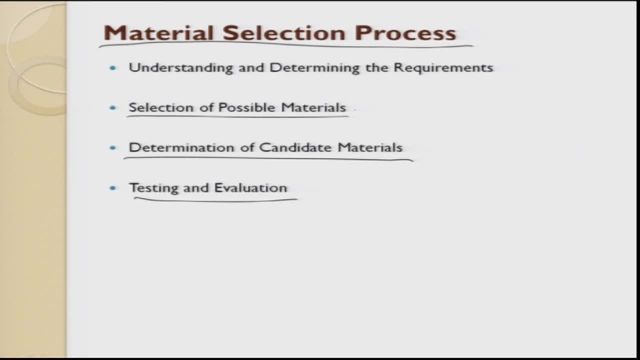 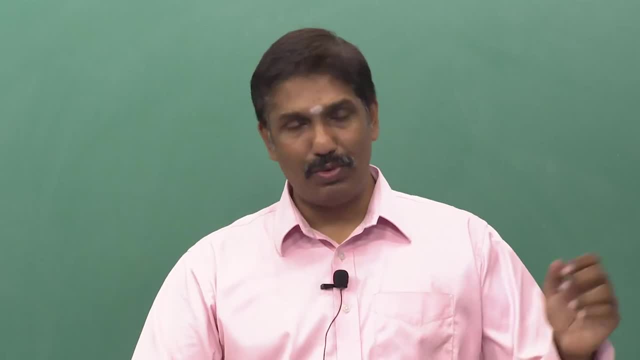 means to say you choose, only polymer is good. So now in polymer you have 3 classification: thermoset, thermoplast, elastomer. now you decide: no, no, I will use only thermoset. In thermoset, you have polyester, you have epoxy. 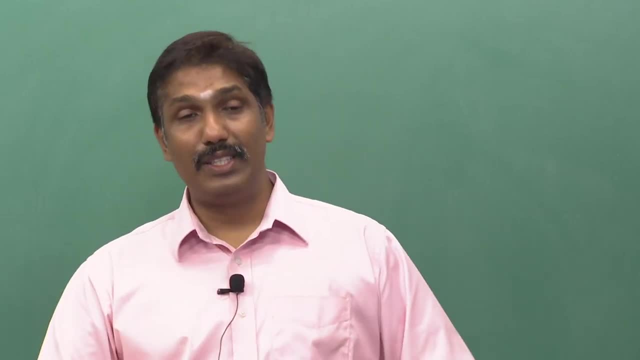 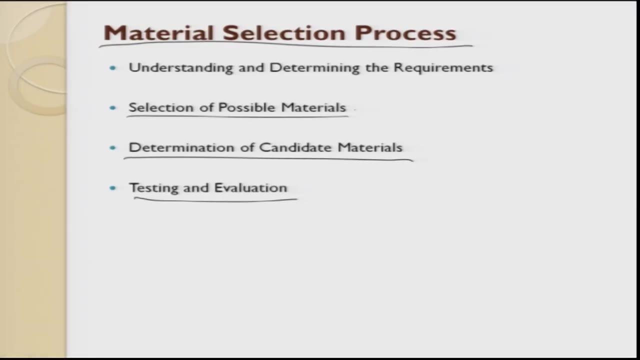 you have vinylester, So you have so many things available. So in this, which one do you choose? And again, after choosing it, what should be the reinforcement? So those are possible things. Then what you do, You determine the candidate material. So what you do is you cannot go by just by. 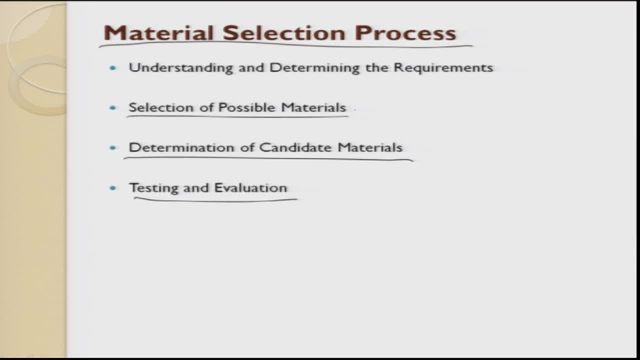 qualitative parameters. You have to convert the qualitative into quantitative values. When you convert into quantitative values, you have each material will have some rank or weightage or whatever it is, So we will determine that. Then what do you do? is we identify a candidate? Then 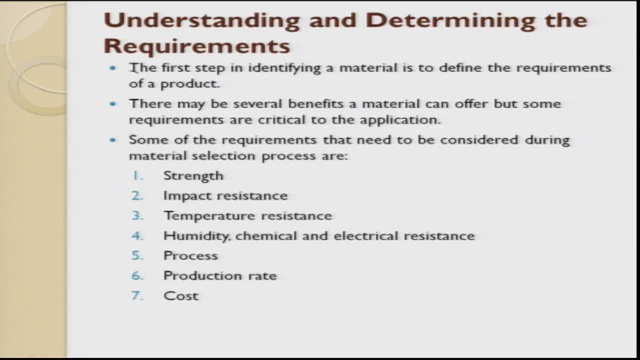 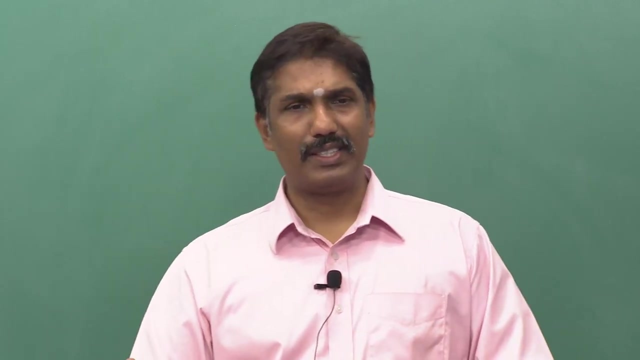 we do testing and evaluation. So the first step is, in identifying a material, is to define the requirements of a product. When you look at a product generally, a product does not undergo only one property or the product never demands only one property. There are many properties. For example, let us take a chair, So in a chair, we always think that. 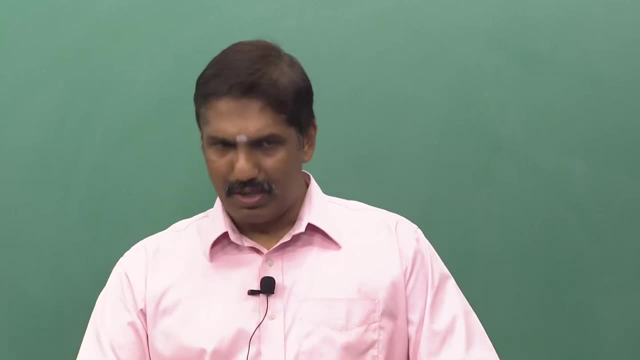 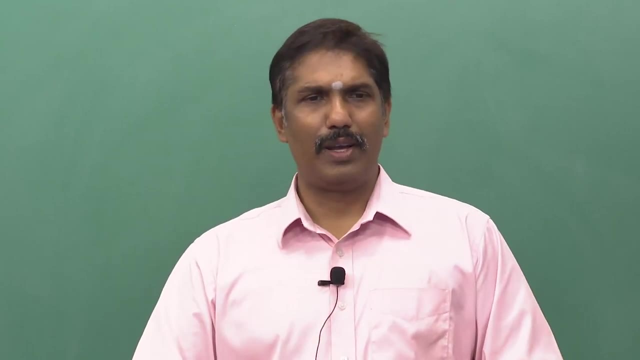 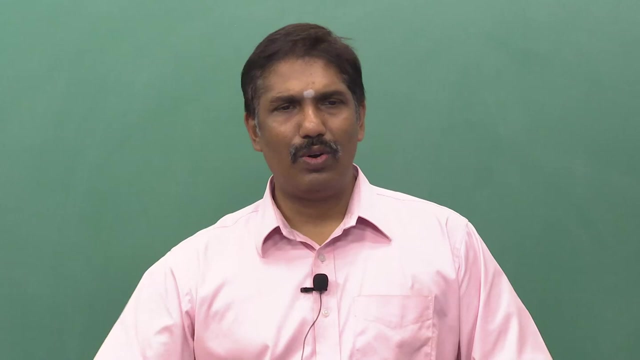 okay, there is compressive load alone, but there is compressive load On top of it. you sit down and slide and move up and down. So when you do it your your hip goes sliding. So the bottom bench where you sit there you have some sliding load coming up and the place where you rest your 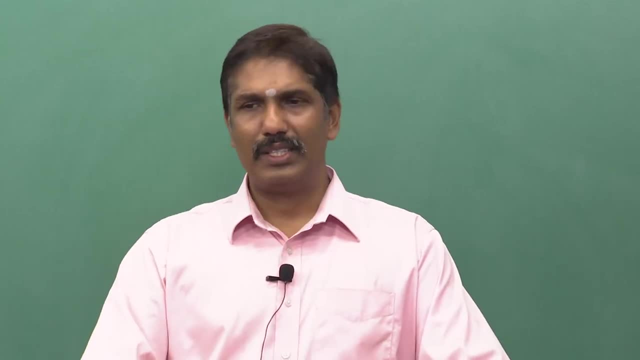 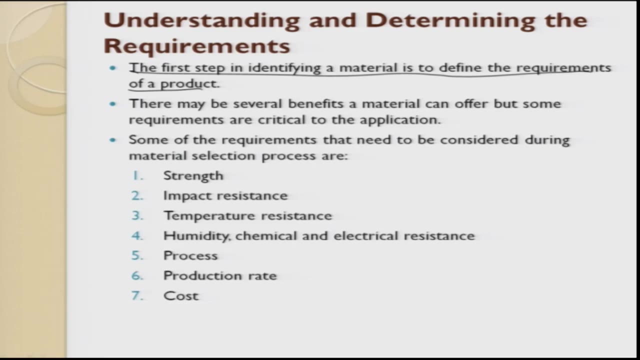 back. there also, you slide. so that is second point. The third thing is roughness. it has to be as smooth as possible. Fourth thing is: when you sit on a chair, we sit as an impact load. When you sit as an impact load, the chair has to take impact load also. so the toughness, 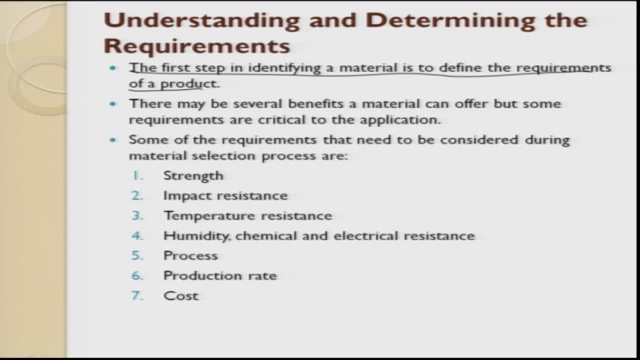 should be high. Now you see, we thought initially it is compressive, but now you see, a list of properties are required. mechanical properties are required from a product, And then, on top of it, the other things are the color, and this color, the texture, all these things. 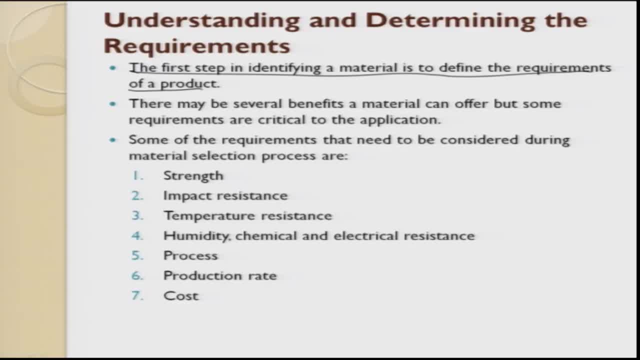 play an important role. The first step is to identify. in identifying a material is to determine the requirement of the product. Once that is done, then the next step becomes very easy. There may be several benefit. there may be several benefits a material can offer, but some requirements are critical to the application. So out of 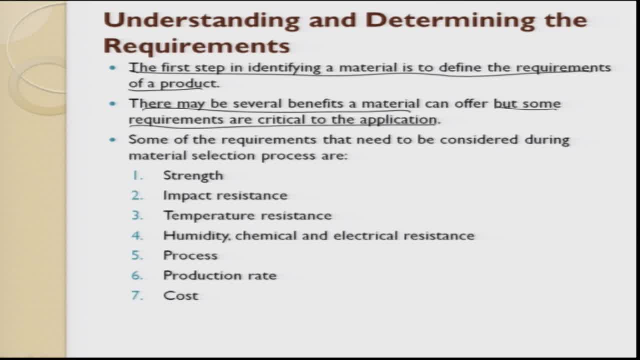 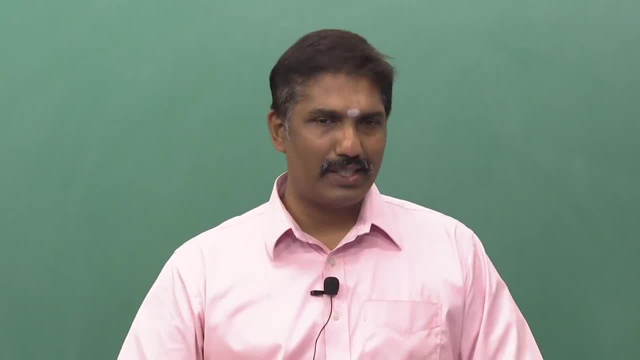 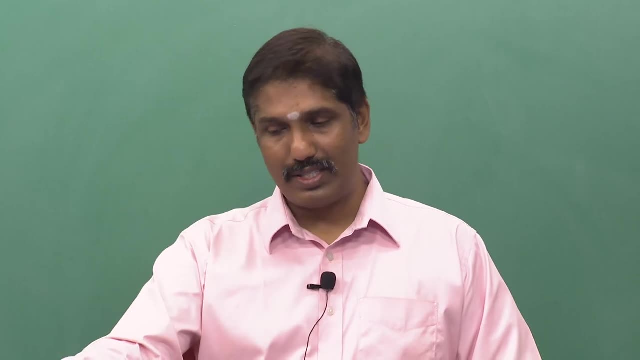 these, so many things. whatever I said for a chair, by and large, a chair has to take a compressive load, it has to distribute the loads between the four legs and it has to have impact load. So this is very important. so, first, what you do, you will listed down. 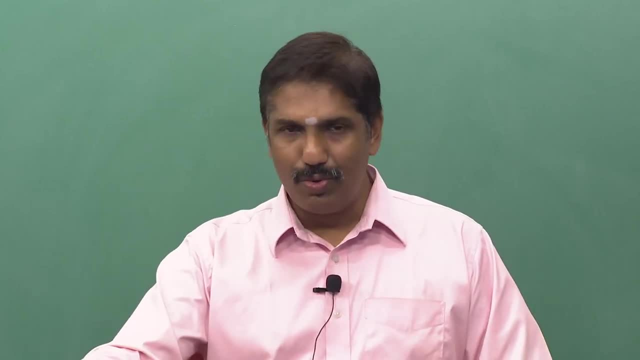 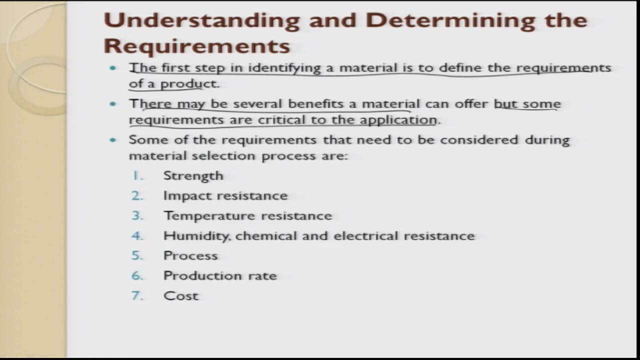 all the properties, what you want from a product. Then you picked up the most critical ones and then you try to solve the most critical ones. so they are called as primary ratio, Primary ratio- requirements, and there are something called as secondary requirements. Secondary requirements we will try to accommodate but we will not give them more weightage. 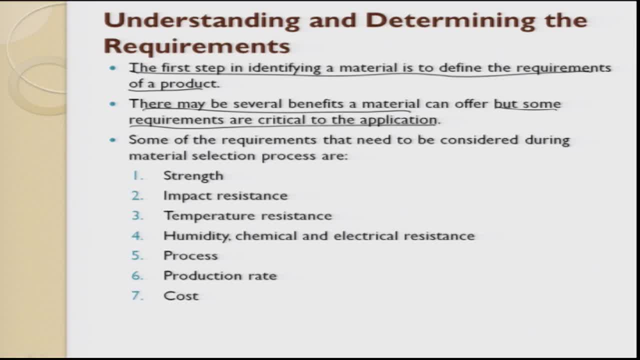 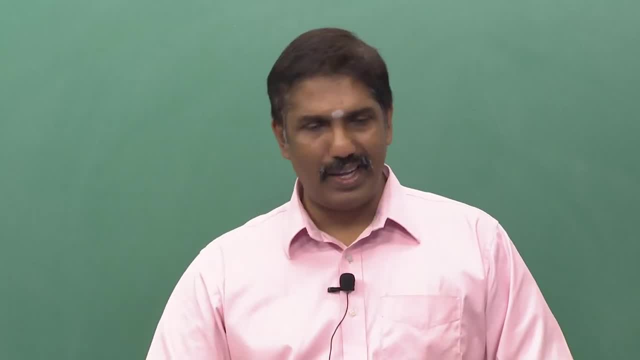 Suppose you do not do this analysis, in industrial engineering term they do something called as ABC analysis. So if you do not do this ABC analysis, we will try to take a property which is very trivial or a secondary property and start giving more weightage for them. but ultimately the customer 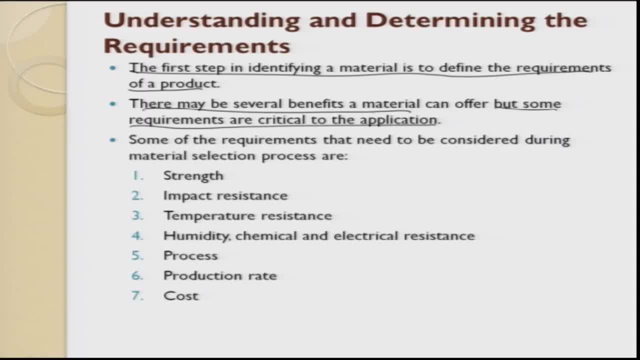 will not be happy. So there are. there may be several benefits a material can offer, but only critical applications. you should look and choose a material. Some of the requirements that need to be considered I am listing down: majority is mechanical, then it is environmental, one is strength. 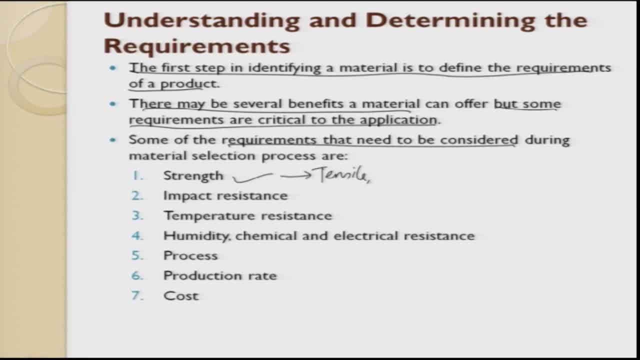 What are the strength? it can be tensile, it can be compressive, it can be shear right and it can. It can be shear, etcetera. Impact resistance: as I said, it is very, very important. So then it is thermal resistance. this is what I was telling in the last class about service. 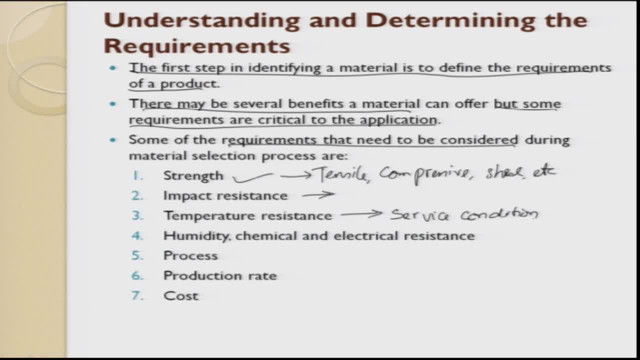 condition. What is the ambience it is present. in which ambience? it is present so that it is expected to perform. Then comes humidity. See the relative humidity in certain parts of the country. You can see it varies from it. the humidity varies from 10 percent. it goes up to 95 percent. 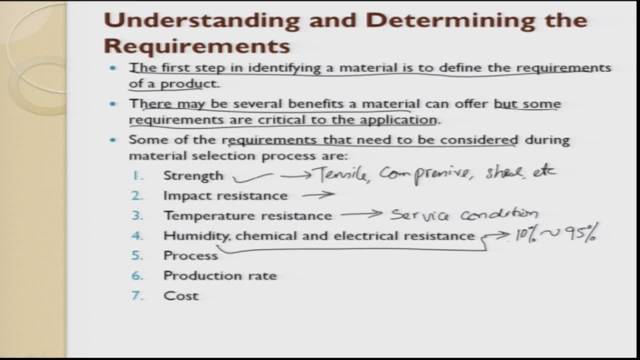 So you see so much of water in the atmosphere. so your your work piece your product should not observe. Then on top of it, chemical and then electrical. So chemical is corrosive environment, electric is- sometimes we use it for insulation properties also. So this process is directly process, production rate and cost- these three are interlinked.